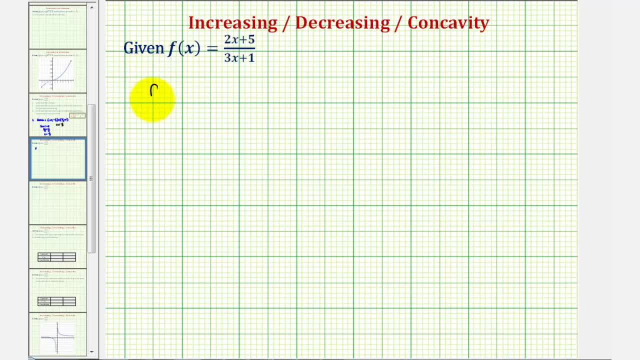 in order to find our derivative here. So f prime of x would be equal to. we'll begin with the denominator, which would be the denominator squared. Our numerator is going to be: is going to be the denominator times the derivative of the numerator, minus the numerator. 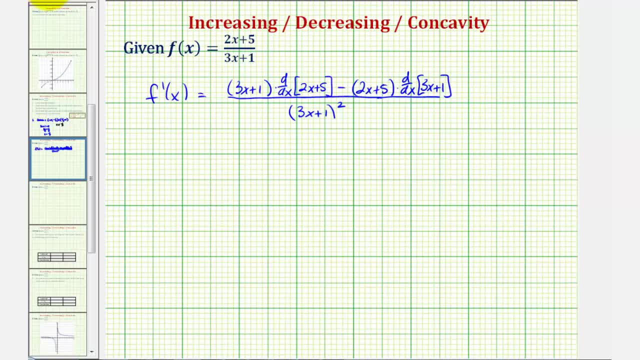 times the derivative of the denominator. So now we'll find the derivative here and here and here And simplify. Our denominator is going to stay the same. The derivative of 2x plus 5 would just be 2.. So we'll have 2 times the quantity, 3x plus 1,. 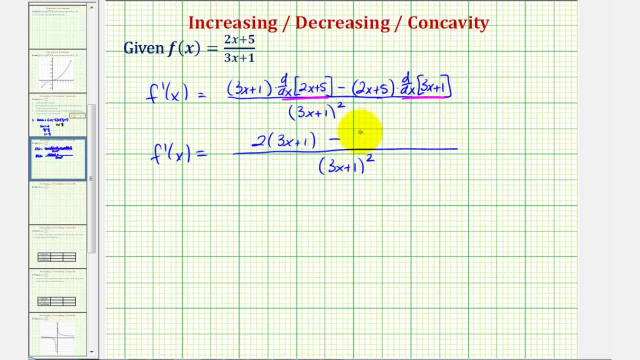 minus, the derivative of 3x plus 1 is 3.. So we'd have minus 3 times the quantity 2x plus 5.. Let's go ahead and simplify the numerator. If we distribute, we'd have 6x plus 2,. 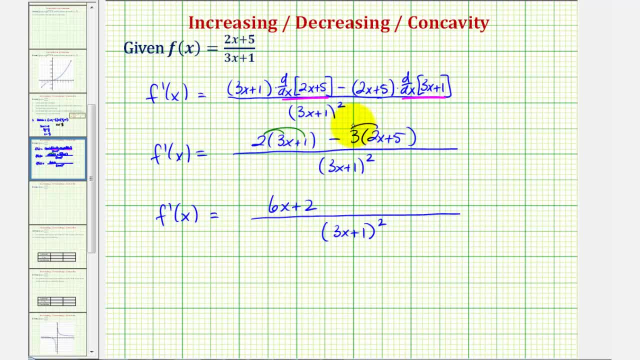 here we'll put differentiateで 3.. So we would have minus 6x minus 15.. Well, 6x minus 6x is zero, and we have 2 minus 15, that's negative 13, divided by the quantity 3x plus 1 to the second. 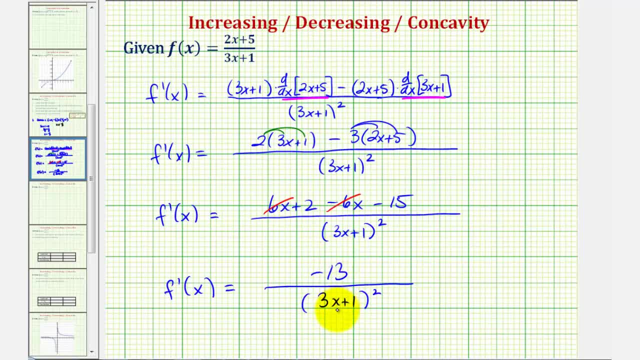 And again the critical numbers occur where this function is equal to zero or undefined. Well, notice how the numerator is a constant, so this will never equal zero. Notice how it is undefined when we have division by zero, or when the quantity three x plus one equals zero. 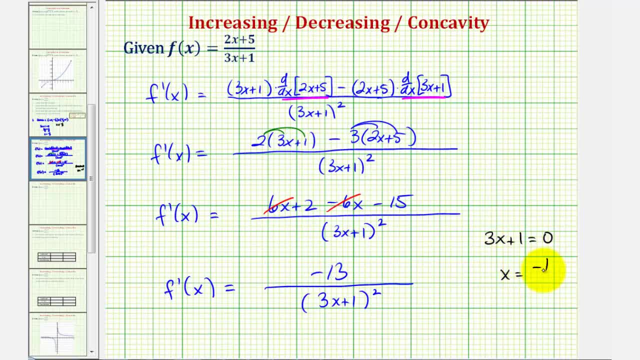 If we solve this for x, just like before, we'd have x equals negative 1, 3rd. This is also the same value where the function is undefined, and we do have to consider this value when determining the sign of the first derivative. It could change signs to the left and right. 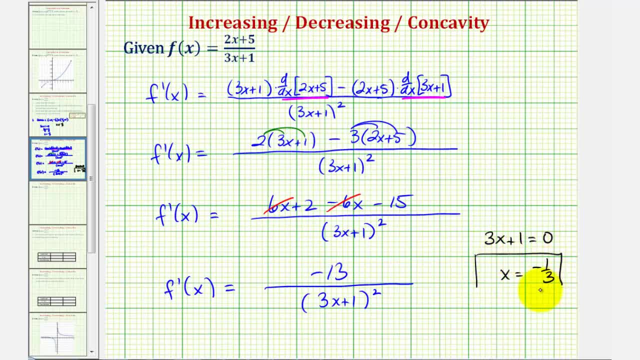 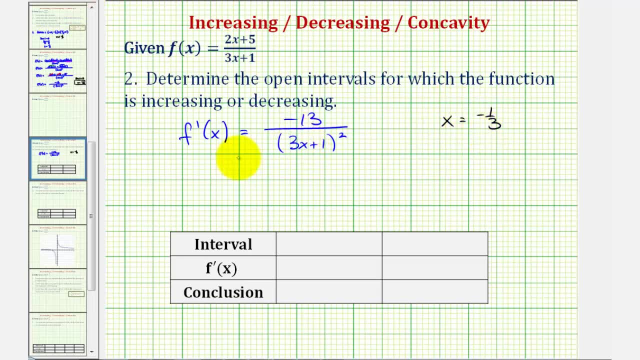 of negative 1- 3rd. So now let's go ahead and set up the intervals to test the sign of the first derivative, Because our domain was all real numbers, except x, equals negative 1- 3rd, because the domain of the function was all real numbers. 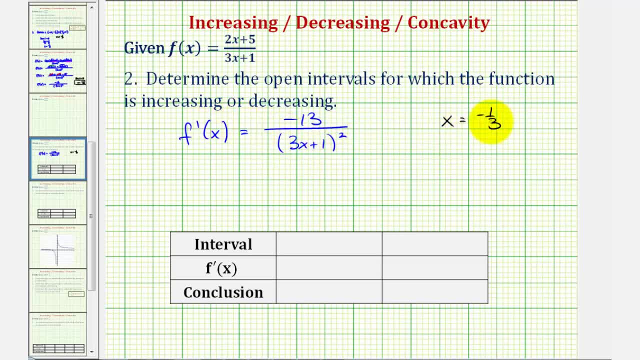 except negative 1- 3rd, and the first derivative is undefined at negative 1- 3rd. our two intervals to test will be from negative infinity to negative 1- 3rd and the open interval from negative 1- 3rd to infinity. 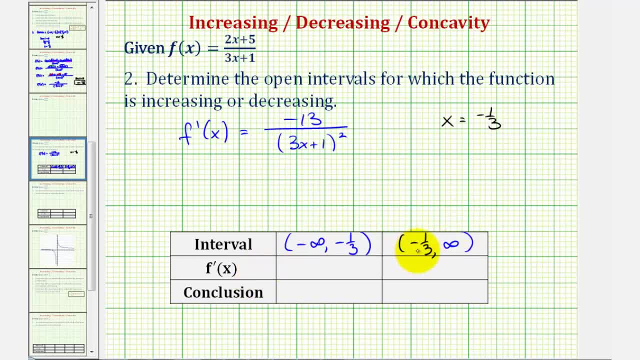 So now we'll test the sign of the first derivative in each of these intervals to determine if the function is increasing or decreasing on that interval. So for this first interval let's go ahead and test. x equals negative one, So f prime of negative one would be negative 13. 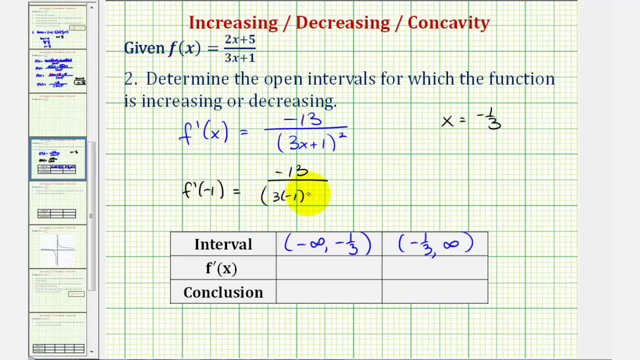 divided by three times negative, one plus one. We don't have to find the exact value, We just have to determine if this is going to be positive or negative And notice how we'd have a negative divided by a positive value and therefore this is going to be negative or less than zero. 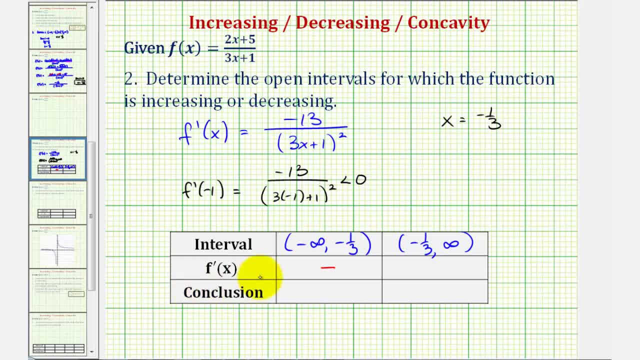 So the first derivative is negative over this entire interval and therefore the function is decreasing over this entire interval. And now for the second interval. let's test: x equals one, So f prime of one would be equal to- again negative 13 divided by the quantity. 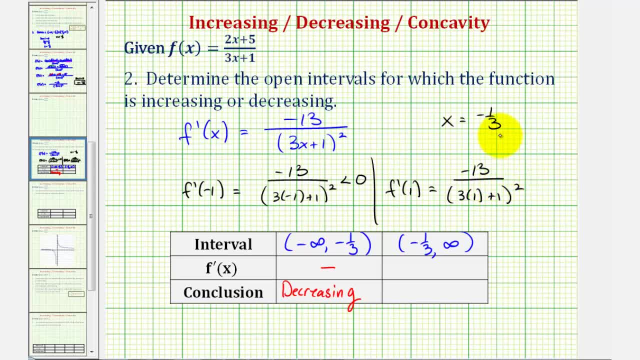 three times one plus one squared Again, we'd have a negative divided by a positive, which is negative or less than zero, and therefore the first derivative is negative over this entire interval. So again, the function is decreasing over this entire interval. 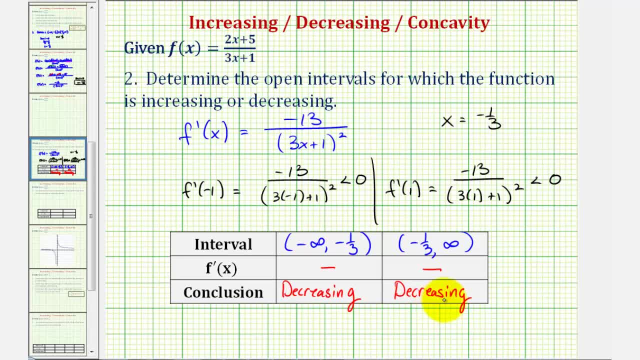 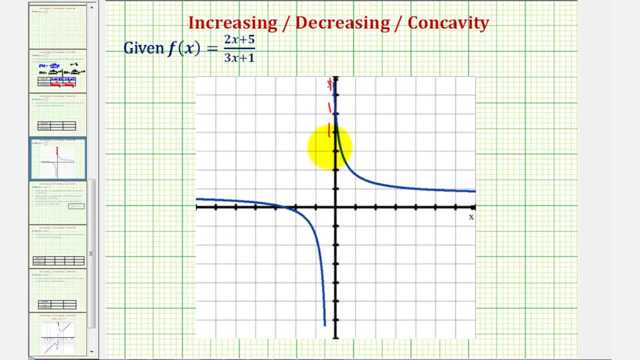 which means the function is decreasing over its entire domain. Let's go ahead and check this on the graph. Notice that x equals negative one-third. we have a vertical asymptote And on the left, or on the interval from negative infinity to negative one-third, 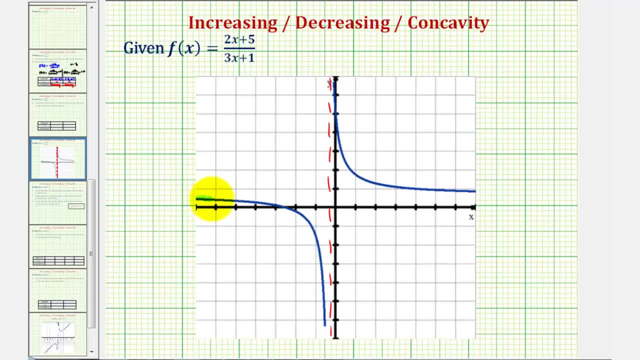 notice how the function is decreasing as x increases or as y decreases, or as we move from left to right- we're going downhill- And also on the right side, or on the open interval from negative one-third to positive infinity. again, as x increases, the y values decrease. 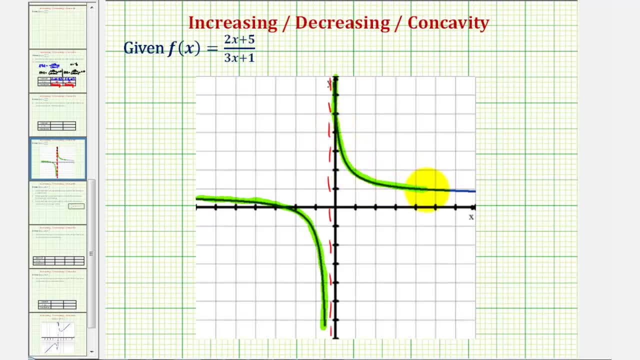 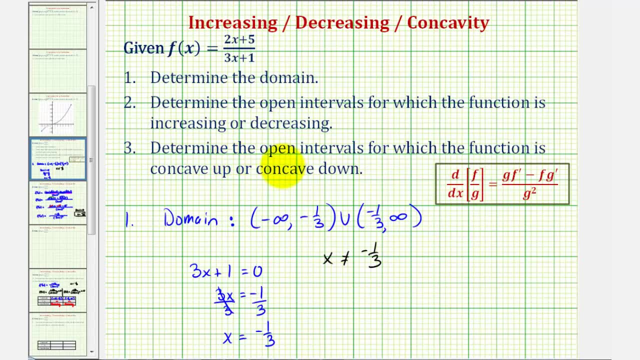 or, as we move from left to right, the function is going downhill. So this verifies the function is decreasing over its entire domain. And now for the third part. we're going to determine the intervals for which the function is concave up or down. 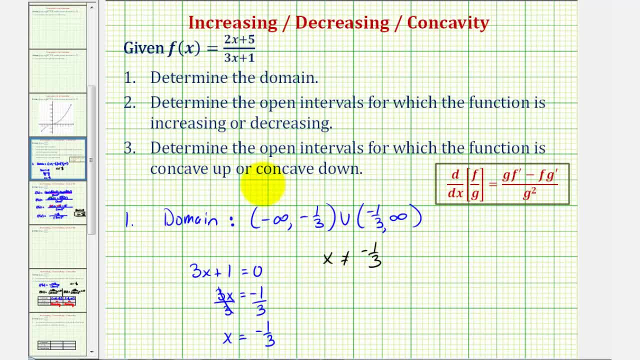 A function is concave up when the second term, the second derivative, is positive, and a function is concave down when the second derivative is negative. So to determine the concavity, we begin by determining where the second derivative is undefined or equal to zero. 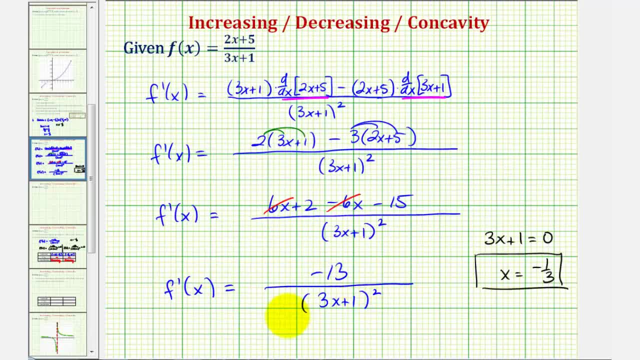 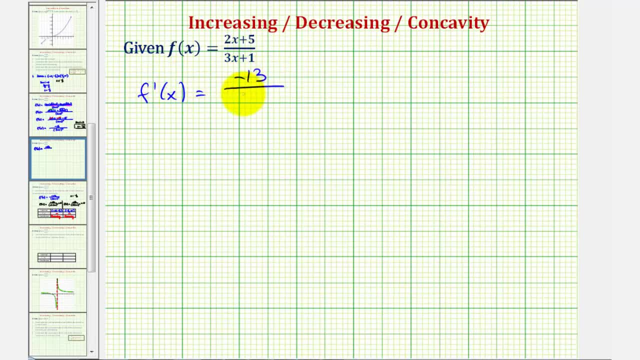 So to find the second derivative, we'll find the derivative of the first derivative. So the first derivative was equal to negative 13 divided by the quantity three x plus one. to the second, Let's go ahead and write this as negative 13 times the quantity three x plus one. 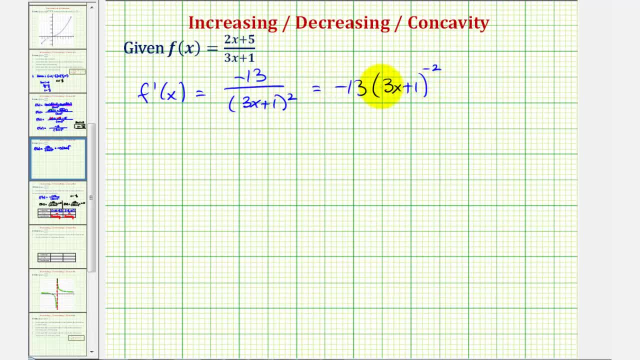 raised to the power of negative two. This way we don't have to apply the quotient rule again, We can just apply the extended power rule. So the second derivative function would be equal to. we do have to apply the chain rule here. 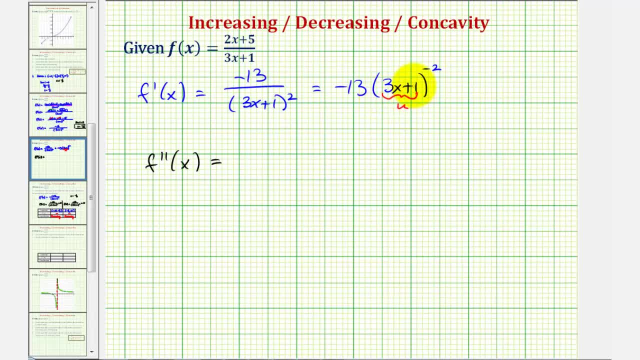 where the inner function three x plus one, we can let it be equal to u. So we can think of this as negative 13. u to the negative two, which means to find the derivative. we would multiply it by negative two, that'd be 26.. 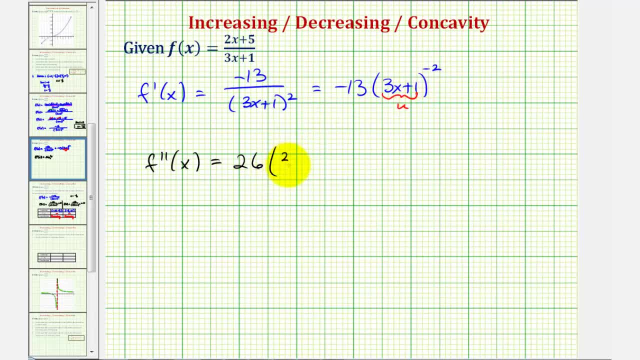 And then we'd have u to the negative three, which is really the quantity three x plus one, to the negative three times u prime, which here, the derivative of three x plus one would just be three. So our second derivative is going to be: 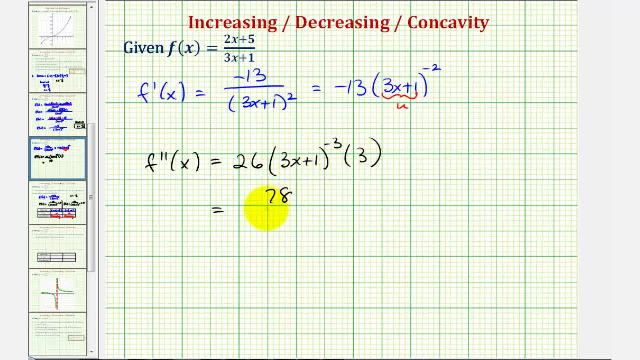 26 times three, that's 78, divided by the quantity three x plus one to the positive three power. If we move this to the denominator, it changes the sign of the exponent. But once again, notice how the second derivative is never going to be equal to zero. 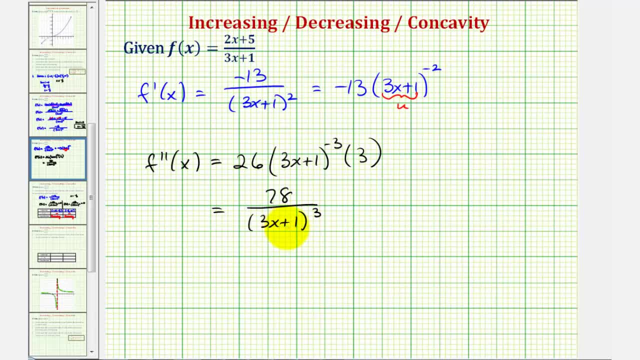 because we have a constant in the numerator. So it's only going to be undefined when the base of three x plus one is equal to zero. Well, just as before, three x plus one is equal to zero when x equals negative 1. 3rd, which is not in the domain, 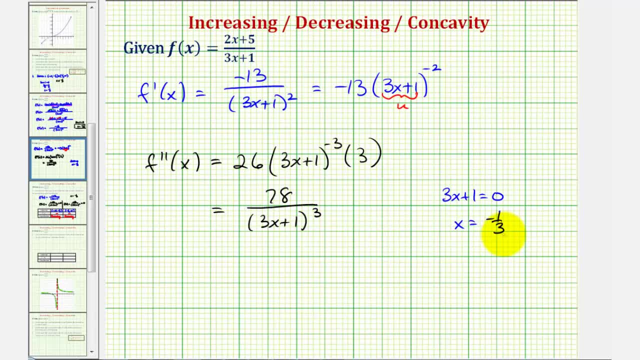 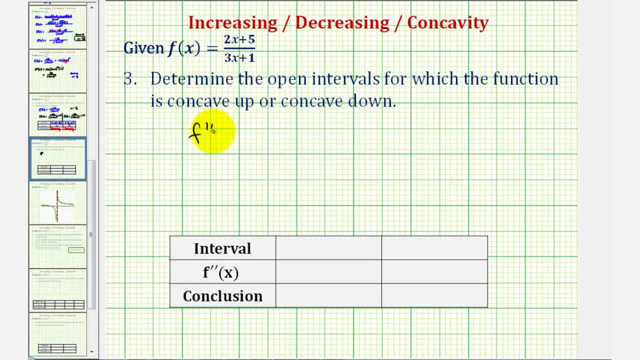 but we'll still use this value to set up the intervals to test for concavity. The function may change concavity to the left and right of negative 1- 3rd. So now, using the second derivative and the fact that it's undefined at x equals negative 1- 3rd. 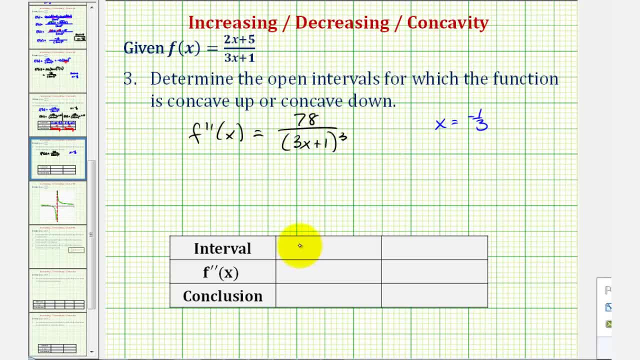 our two intervals once again will be the open interval from negative infinity to negative 1- 3rd and the open interval from negative 1- 3rd to positive infinity. But now, because we're talking about concavity, we'll be testing the sign of the second derivative.